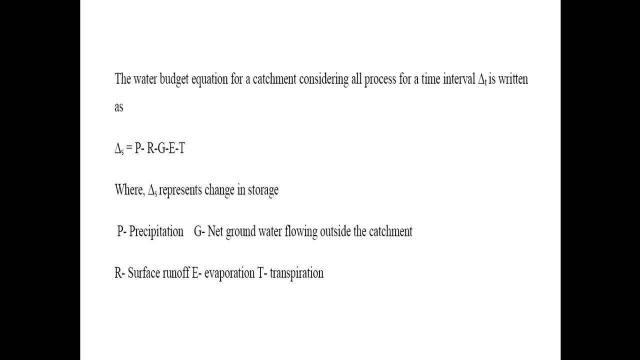 for time interval, delta t is written as: delta s equal to p minus r minus g, minus e minus t. so uh, the water budget equation for any catchment area, uh, including all the processes, or considering all the processes, uh, in a day, in a given time interval, delta t. 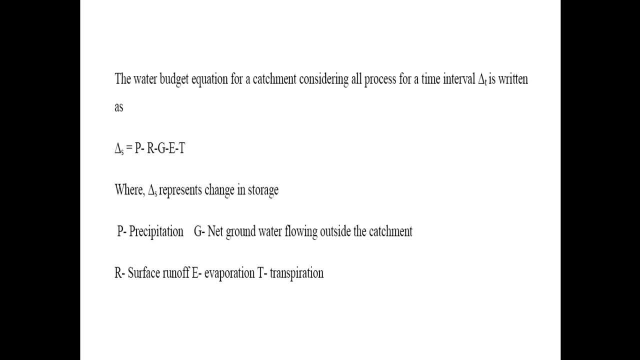 is written as a delta s equal to p minus r minus g minus e minus t. here, delta s represents the change in storage. uh, p is the precipitation, r is the surface runoff, g is the net groundwater flow outside the catchment area, e is the evaporation and t is the transpiration. so in order to get 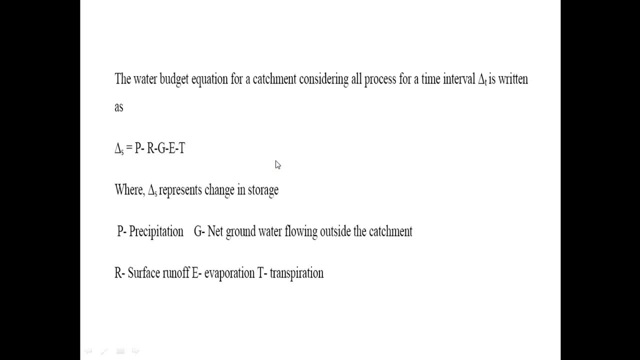 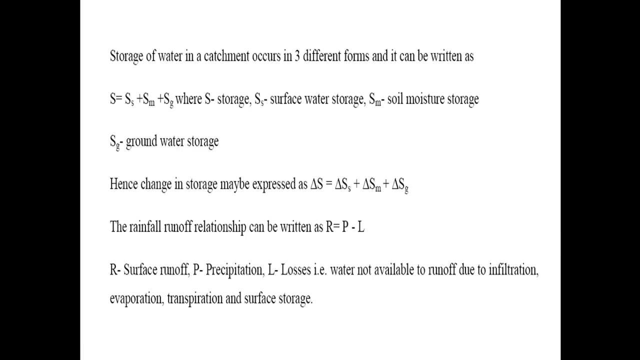 the delta s. that is the change in storage. we have to minus the surface runoff, ground net, groundwater flowing outside the catchment, evaporation and transpiration from the precipitation and we will get the net change in storage that is delta s. storage of water in a catchment occurs in three different form, and it can be written as s is equal. 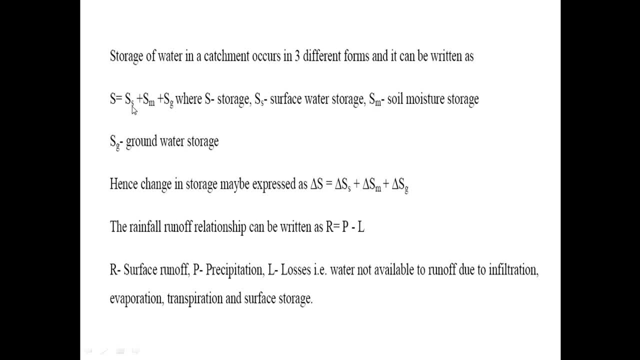 to s, m plus s, m, ss plus sm plus sg, where s is the storage? sm is the surface water storage, sm is the soil moisture storage and sg is the groundwater storage. so, uh, for any catchment, uh this uh the water storage form, uh the water storage occurs in these three forms. hence, uh change in storage may be expressed. 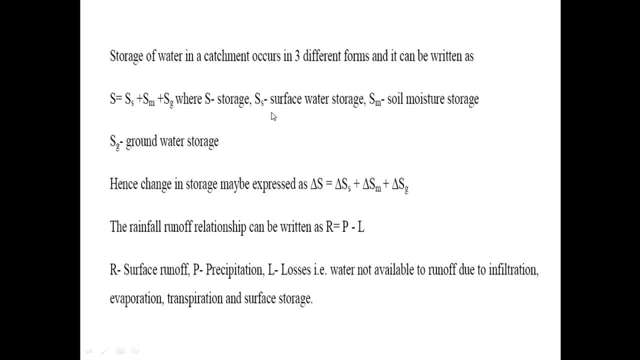 as delta s is equal to delta ss plus delta sm plus delta sg. so in order to get the change in the storage uh, we denote uh this uh above equation, as delta s equal to delta ss plus delta sm plus delta sg. the rainfall runoff relationship can be written as: r is equal to p minus s. this equation- 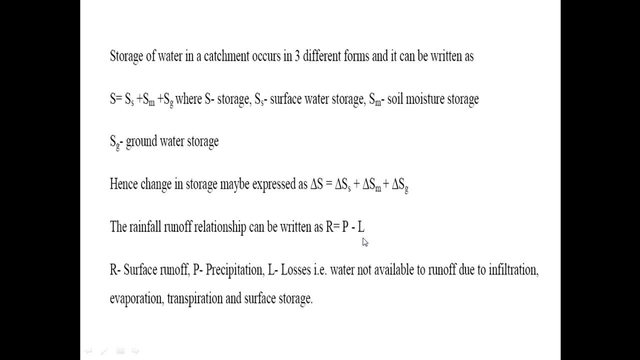 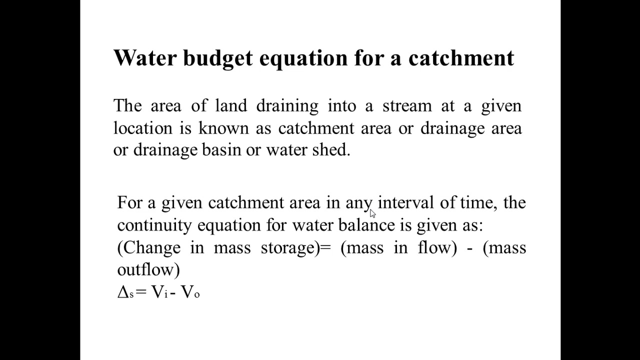 is used for finding uh the relationship between uh rain for all runoff uh. here, r is the uh surface runoff, p is the precipitation and l is the losses. that is, a water not available to runoff due to infiltration, evaporation, transpiration or surface storage. so uh, this is uh known as the water budget equation for a given catchment area, or also 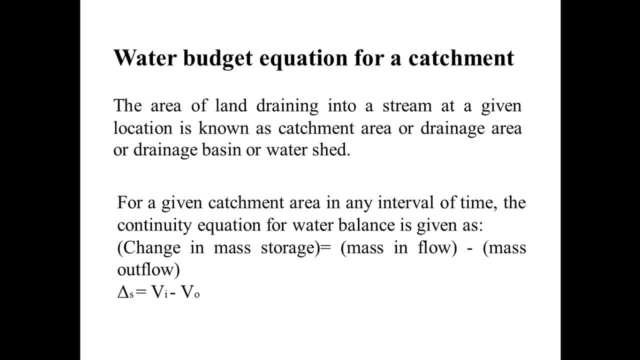 known as the water balance equation. uh for a given catchment area, uh, this can then cards cashment area is: who have drainage area? be caitain drainage basin. because water uh time interval continuity equation for water balance is change in mass storage equal to mass inflow minus outflow means change in mass. 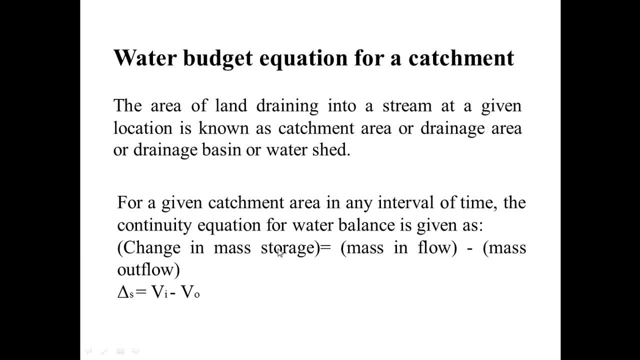 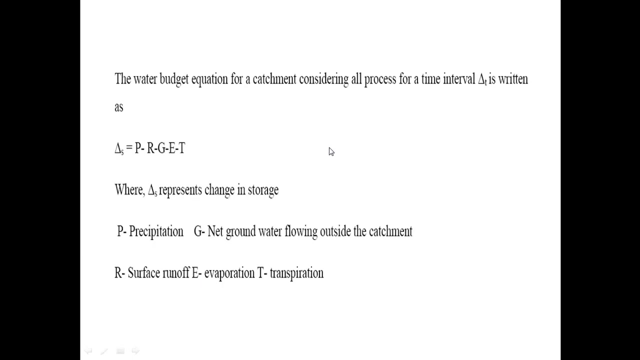 storage is equal to change in mass inflow minus outflow. so we will get the change in mass, change in mass storage. we denote as delta s mass inflow. we denote as vi and mass outflow to be v0. the water budget equation considering all processes for a given time interval: delta T: 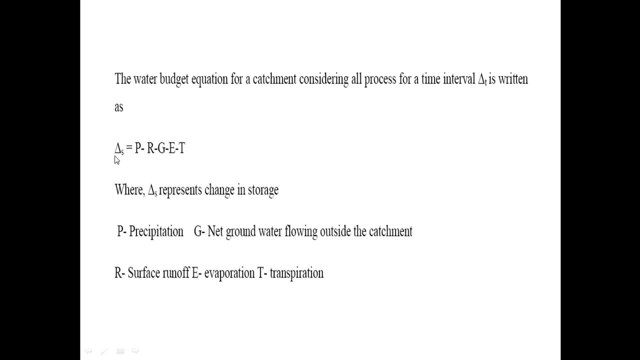 for any catchment area, we write as: delta s is equal to P minus R minus G, minus E minus T. for any catchment area, we write as: delta S is equal to P minus R minus G, minus E minus T. P is net precipitation, R is surface runoff, G is net groundwater flowing outside the catchment area, E is evaporation and T is transpiration. 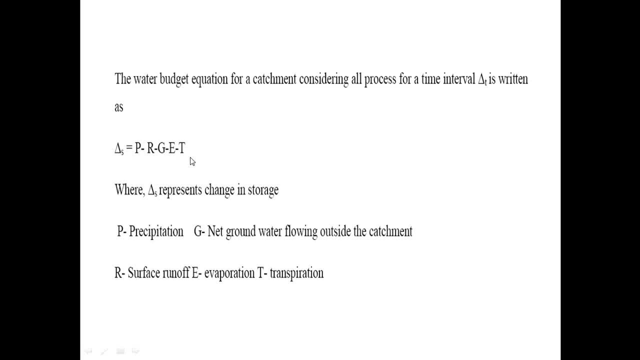 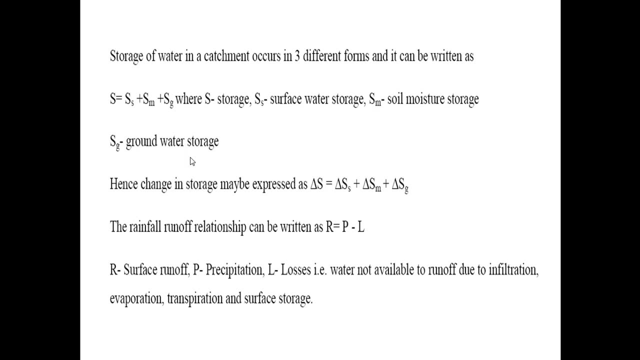 Delta. S represents the change in storage. The storage of water in any catchment has three different forms: S is equal to Ss plus Sm plus Sg. S is total storage, Ss is surface water storage, Sm is soil moisture storage and G is groundwater storage. 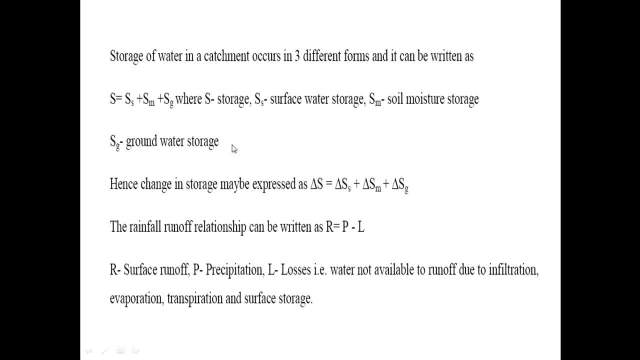 The change in storage is expressed as: delta S is equal to delta Ss plus delta Sm plus delta Sg. The rainfall runoff relationship is written as: R is equal to P minus L, R is surface runoff, P is precipitation and L is losses. 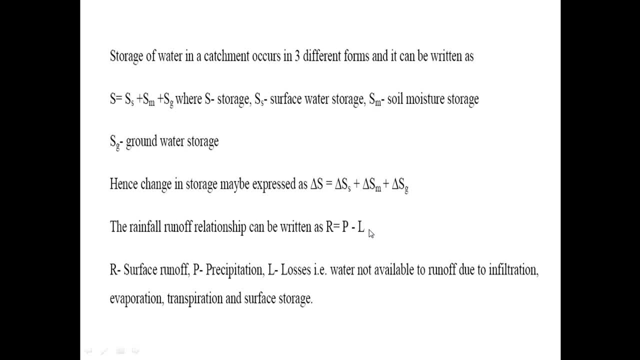 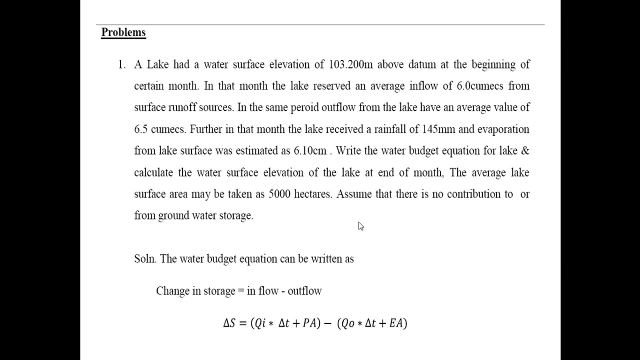 The losses occur when water is not available. The runoff is due to infiltration, evaporation, transpiration or surface storage. That means the water that is not available for runoff is considered as losses. Let's solve the problem. So we have problems. 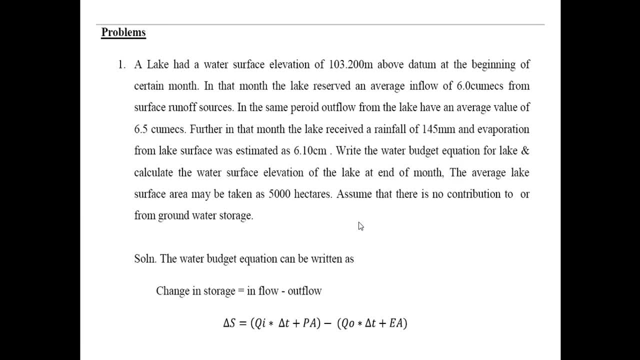 Number one. A lake had a water surface elevation of 103.200 meters above the data map At the beginning of a certain month. in that month, the lake reserved an average inflow of 6 cubic meters from surface runoff sources. In the same period, outflows from the lake have an average value of 6.5 cubic meters. 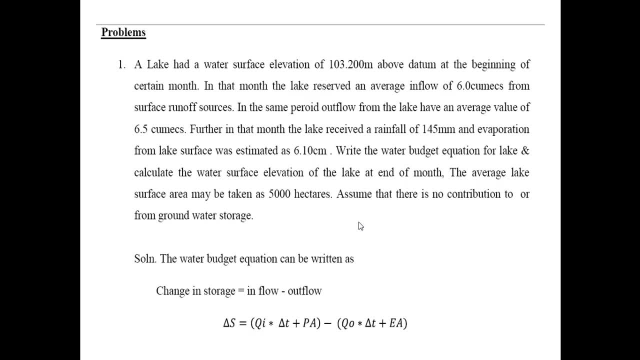 Further in that month, the lake received a rainfall of 145 millimeters and evaporation from the lake surface was estimated as 6.10 centimeters. We will write the water budget equation for the lake and calculate the water surface elevation of the lake at the end of the month. 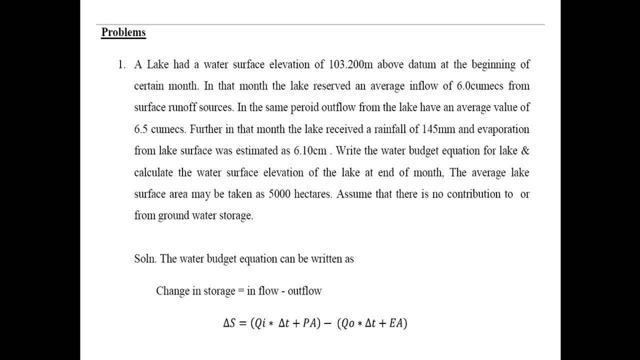 The average lake surface area may be taken as 5,000 hectares, Assume that there is no contribution to or from groundwater storage. So in this problem we will calculate the water surface elevation of the lake at the end of the month. Also, we will write the water budget equation for the lake. 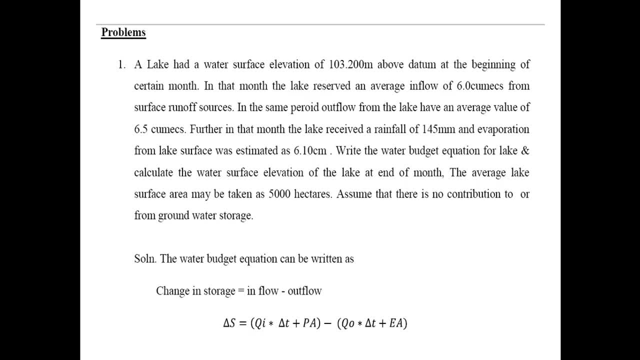 The given data is: the water surface elevation is given, which is 103.200 meters above the data in the beginning of a certain month. Also, the lake reserved average inflow is given, which is 6 cubic, that is, 6 cubic meters per second from the surface runoff sources. 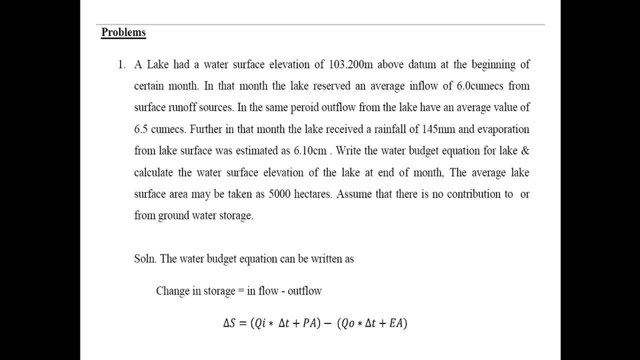 Also in the same period, outflows from the lake have an average value of 6.5 cubic meters per second. In that month, further, the lake received 145 millimeters of rainfall, And in that period, evaporation from the lake surface was estimated to 6.10 centimeters. 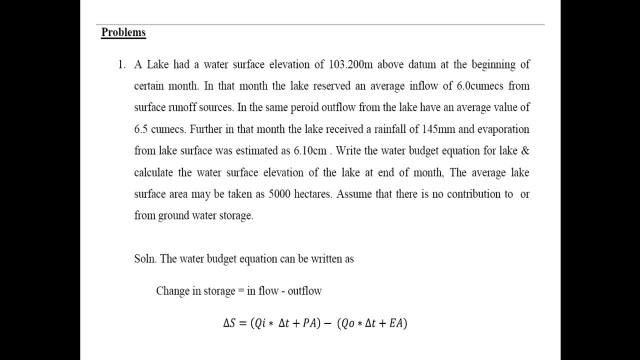 The average surface area to be taken for the lake is 5,000 hectares. We have to assume that there is no contribution to or from groundwater storage. So first of all, we will write the water budget equation And it can be written as: change in storage is equal to inflow minus outflow. 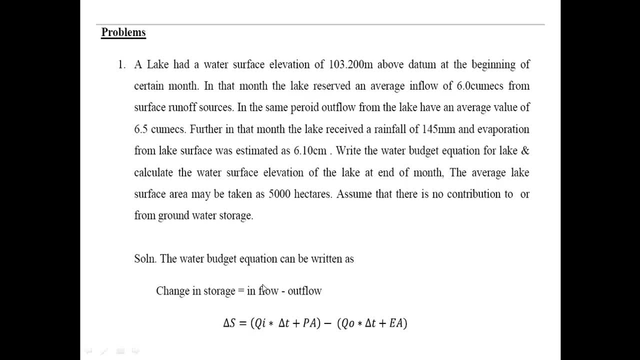 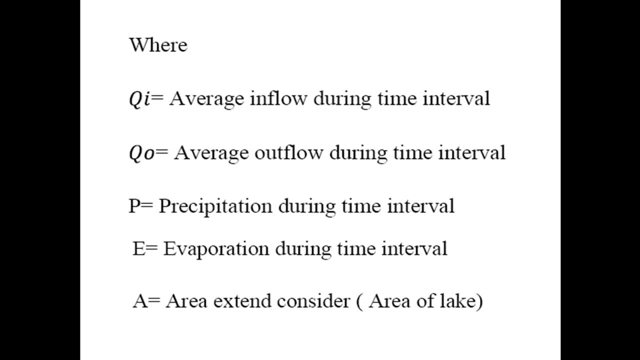 So change in storage is denoted by delta S Inflow. is QI into delta T plus P into A minus Q naught into delta T plus EA Means that is QI is the average inflow during the time interval, Q- naught is the average outflow during the time interval. 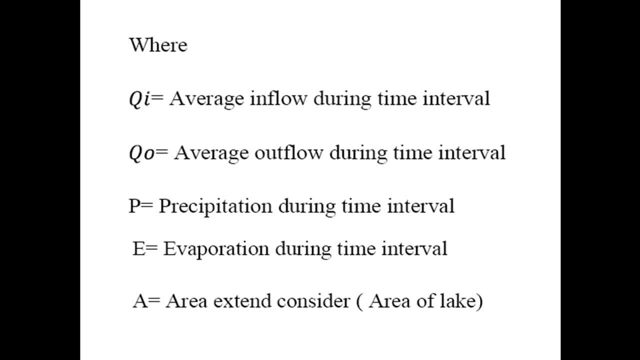 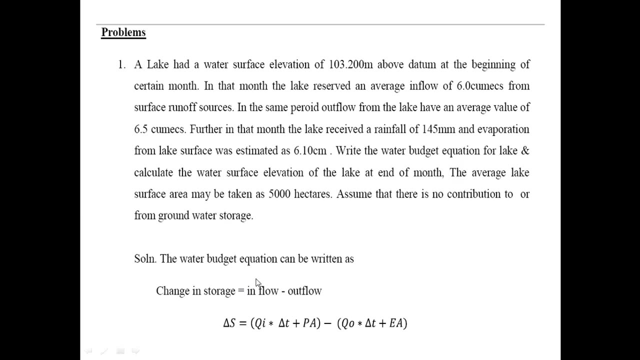 P is the precipitation during time interval, E is the evaporation during time interval And A is the area extended considered, that is, area of the lake. So these are the different terms which are explained here. So QI, which is the 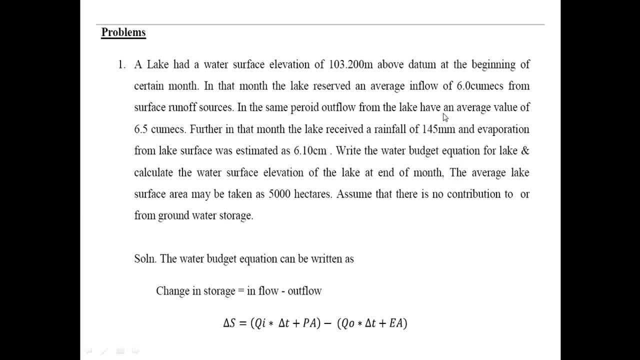 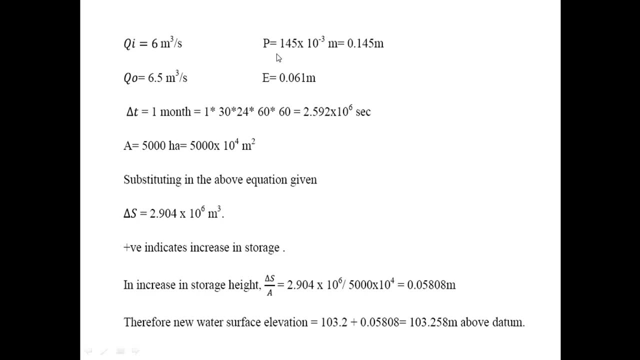 Average inflow during the time interval is given, that is 6 cubic meters per second. P. that is the average. Sorry, the rainfall that is received during that month is 145 centimeters, So that is equal to 0.145 meters. 145 centimeters is equal to 0.145 meters. In fact, that is Millimeter. sorry, I told that it is 145 centimeters. It is 145 millimeters, So 145 millimeters is equal to 0.145 meters. 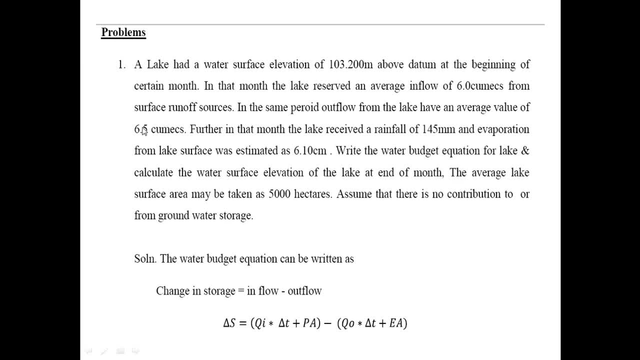 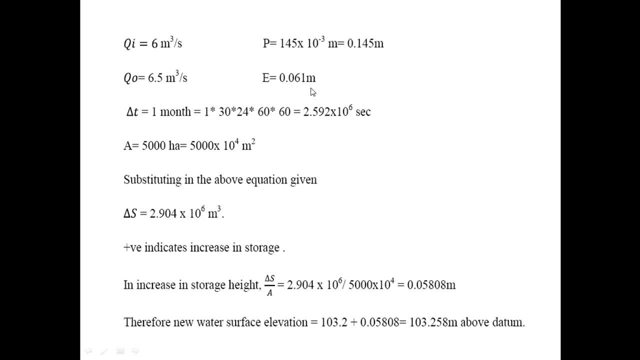 Q naught is the average outflow during the time interval, And that is equal to 6.5 cubic meters per second, Which is given. E is the evaporation from the lake That is given, which is 6.1 millimeters. 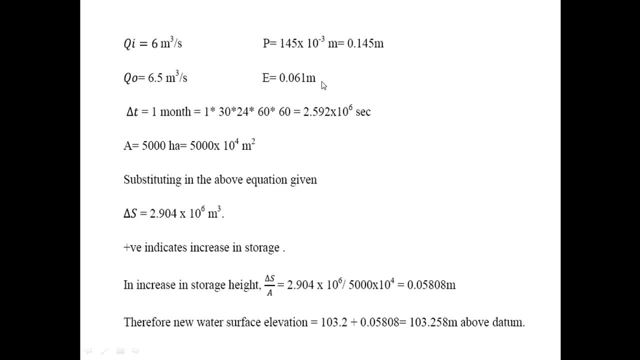 And that is equal to, And that is equal to 0.061 meters Delta t is one month, So that is 1 into 30.. One month have 30 days And one day have. One day is 24 hours. 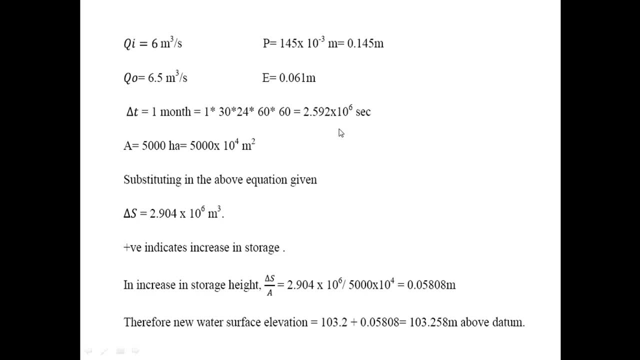 And then one hour is 60 minutes And 60 minutes have 60 seconds. So we will get the total delta t. That is the time in, That is in second. That is 2.592 into 10 to the power 6 seconds. 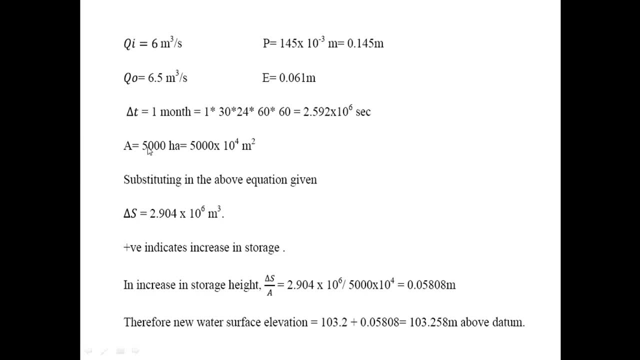 The total area A is equal to 5000 hectares. That is equal to 5000 into 10, to the power 4 square centimeters. Now substituting the values in the Bobb equation, So we will get the total change in storage delta S. 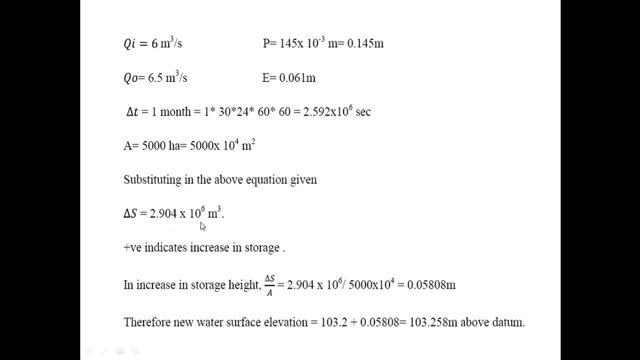 That is equal to 2.904 into 10 to the power 6 cubic meters. The positive sign, The positive value, indicates that the increase in storage, That we have an increase in the storage water In increase in storage height, delta S divided by A is equal to 2.904 into 10 to the power 6.. 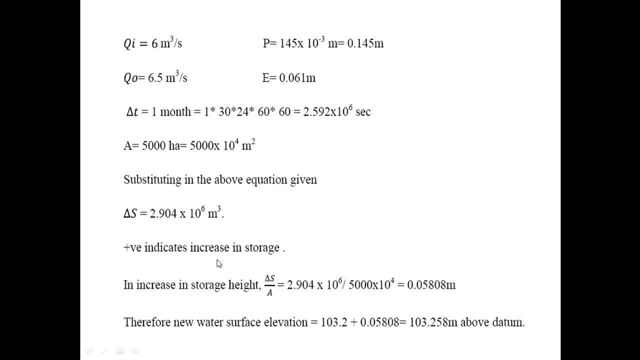 Divided by 5000 into 10 to the power, 4 is equal to 0.05808.. So this much height We have increased. We have increased this much in storage height. So we have the total change in storage. We divided it from the area. 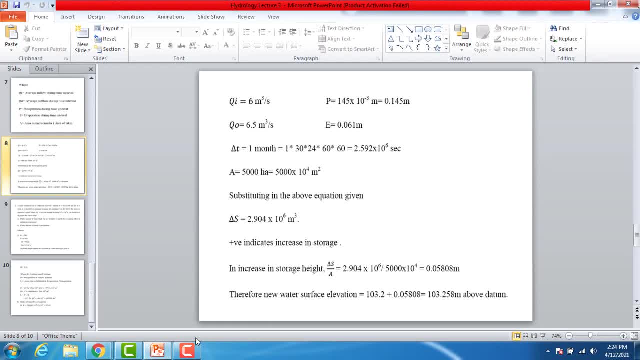 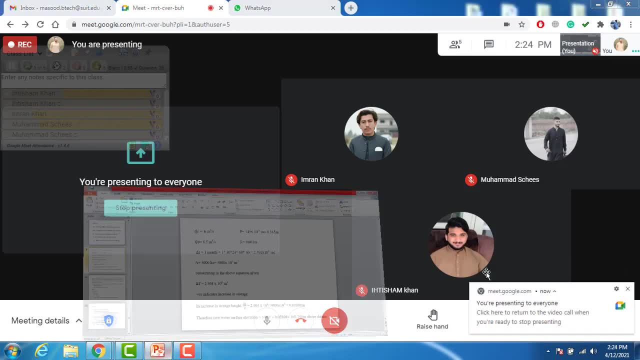 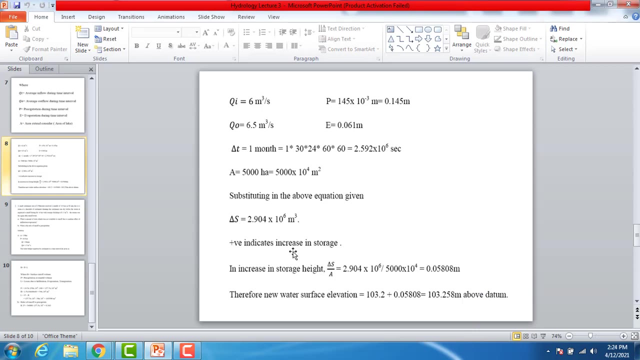 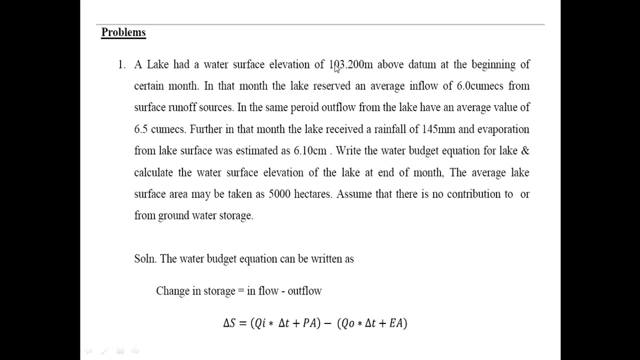 So we have the total value of change in height That we have, After that The new, The new surface water elevation that we have to find. So in order to calculate the new surface elevation, The given surface elevation is 103.200 meters. 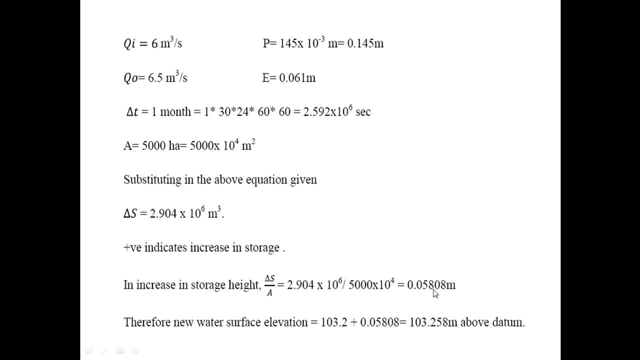 So add 0.05808 with this value And we will get the new water surface elevation, And that is equal to 103.258 meters above the data. So in this way you will calculate the total: The total new surface elevation. 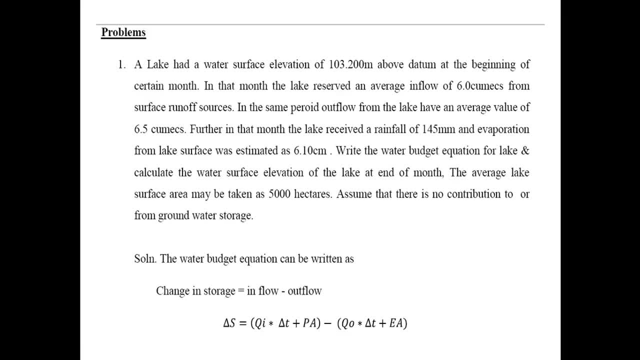 And also write the water budget equation for a given lake. In this problem we have the water elevation given. The water surface elevation of the lake is given, Which is 103.2 meters Above the datum in the beginning of the month. 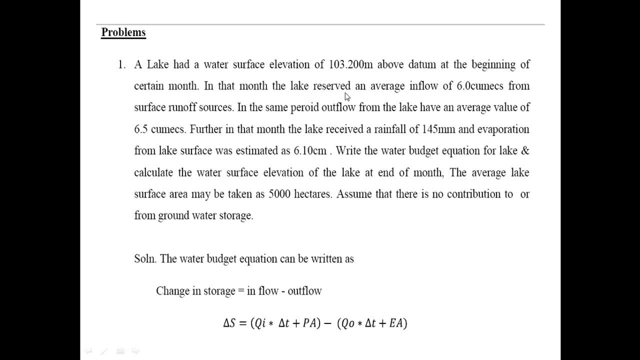 Any certain month In the lake, the reserve, The average inflow is 6 cubic meters per second And from the surface run of sources And the outflow is 6.5 cubic meters per second. In the same month, the rainfall is 145 mm. 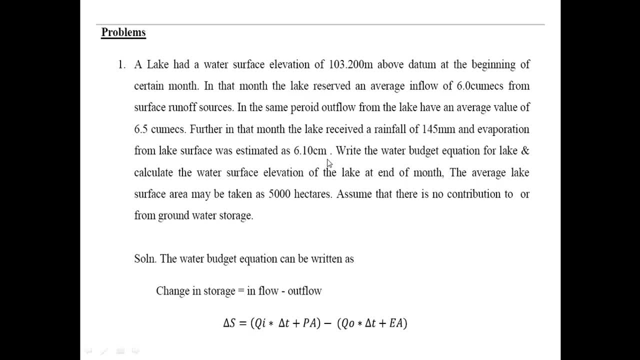 And the operation of the lake is 6.10 centimeters. For this lake we have to write the water budget equation. Along with that we have to find the new water surface elevation at the end of the month. The average lake area is given as 5000 hectares. 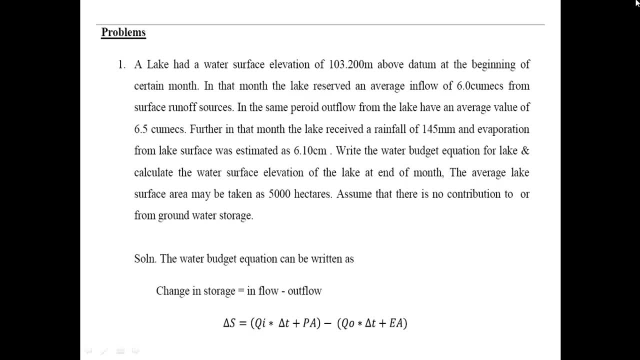 We have to assume that there is no contribution to or from groundwater storage. In other words, there is no contribution to or from groundwater storage in our lake. So we have the water budget equation And we have the change in storage, which is equal to inflow minus outflow. 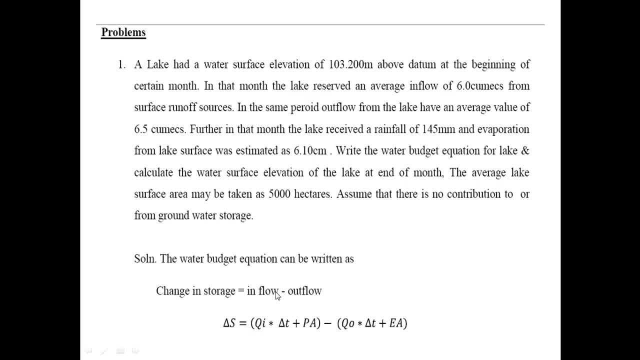 We denote the change in storage as delta s In inflow. we have the inflow of water. In how much time? Along with that, we have the precipitation And we have the area Minus the outflow. Q naught is the outflow. 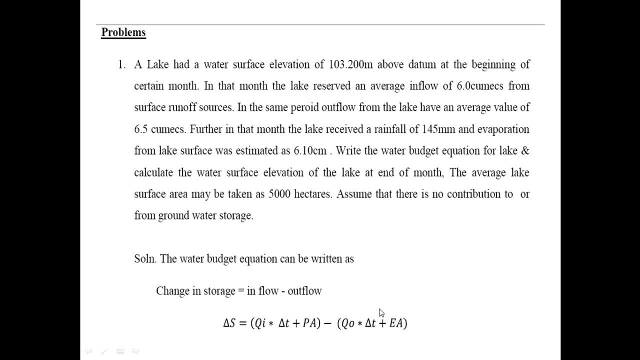 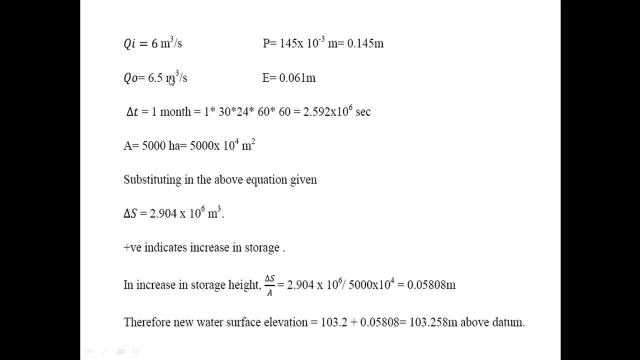 In how much time. This is the evaporation And this is the area. Inflow is equal to 6 cubic meters per second. Outflow is equal to 6.5 cubic meters per second. Precipitation is equal to 0.145 meters. 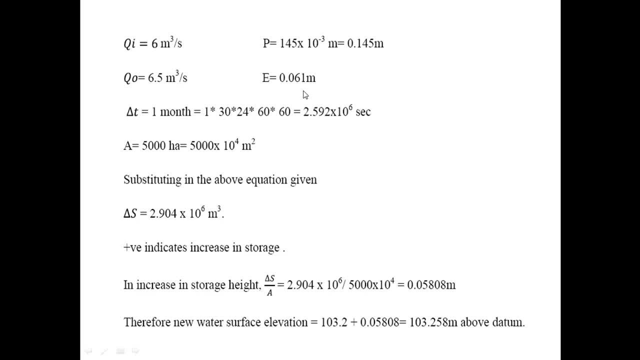 Evaporation is equal to 0.061 meters, Time is equal to 2.592 into 10, to the power of 6 seconds, And the area is equal to 5000 into 10, to the power of 4 square meters. 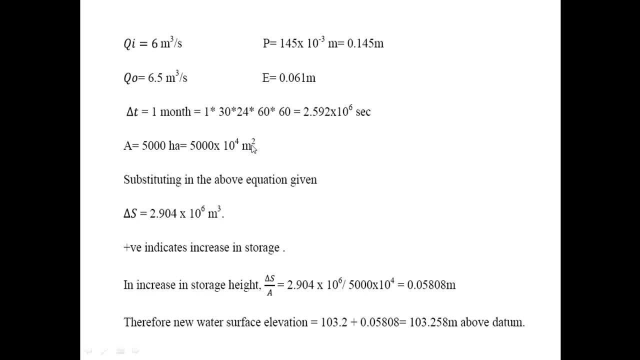 All the values are above and above, So we have to put the value in the budget equation. So we will get the total delta s value, That is equal to 2.904, into 10, to the power of 6 cubic meters per second. 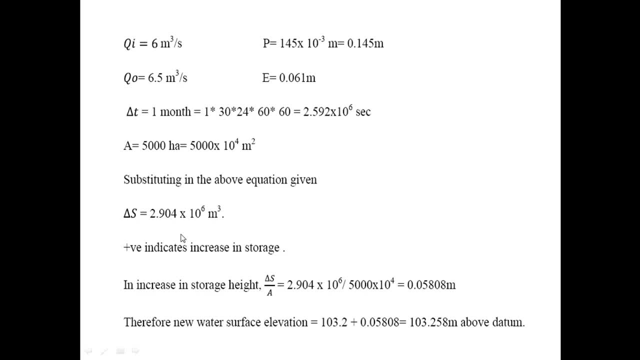 This value is in positive, This means that we have an increase in storage. That is, we have an increase in storage. If this value comes in minus Delta s value, This means that you have a decrease in storage. The total height is according to delta s. 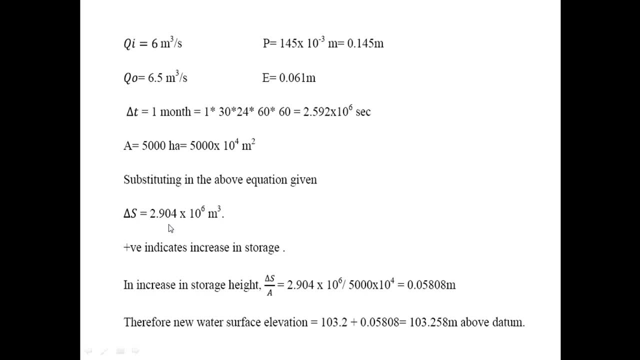 We have to calculate the total height. So to calculate that height you are dividing delta s by the total area, So you will get the increase in storage height. So you have it equal to 0.05808 meters. Okay, So in the question you have been given, 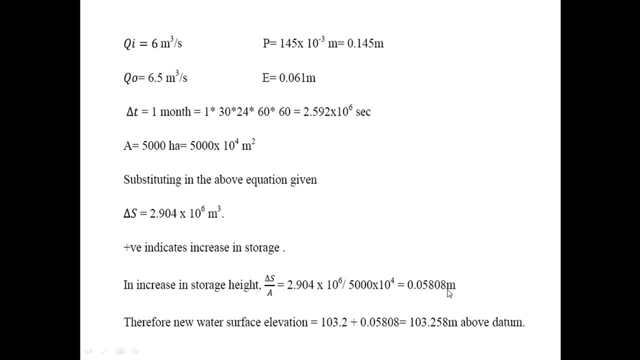 You have to calculate the new surface water elevation at the end of the month. Okay, So given the water surface elevation above the datum line, You have to add it with that, So you will get the new water surface elevation, And that is equal to 103.258 meters above the datum. 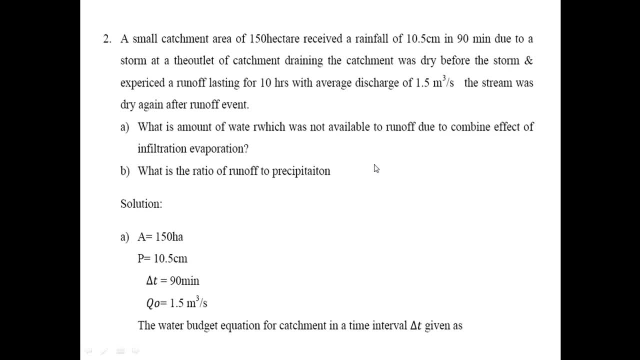 The next example is our statement of. the example is a small catchment area of 150 hectare Receive a rainfall of 10.5. Centimeter in 90 minutes due to a storm at the outlet of a catchment training. The catchment was dry before the storm and experience a runoff lasting for 10 hours with average discharge of 1.5 cubic meters per second. 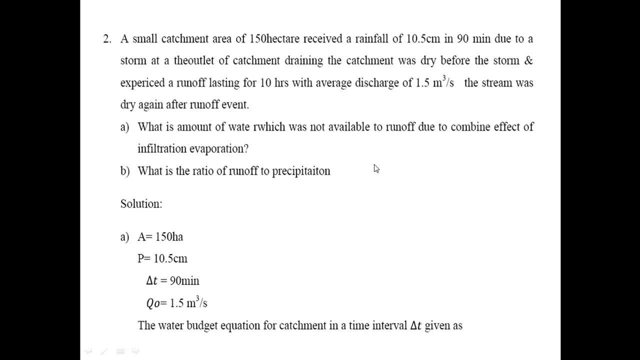 The stream was dry again after runoff. What is the amount of water which was not available for runoff Which are available, Was not available to runoff due to combine effect of infiltration evaporation and be what is the ratio of the runoff to precipitation? So in this example we have to calculate the amount of water which is was not available to runoff due to combine effect of infiltration evaporation. 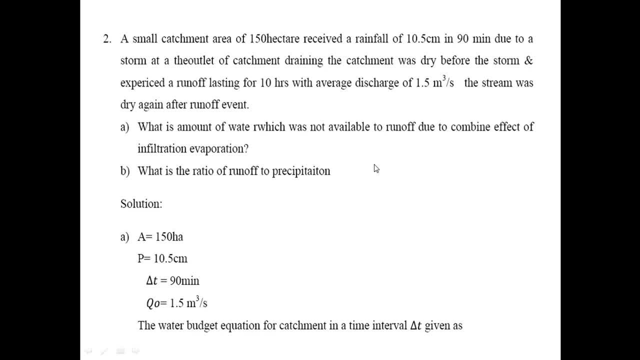 Also, we will have to calculate the ratio of runoff to precipitation. The given area values are: the catchment area is given, which is 1.5.. Centimeter, The area is given, which is 150 hectares. rainfall which received is given 10.5.. 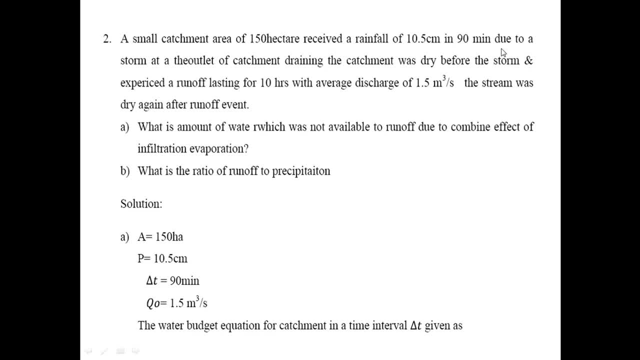 Centimeter at the time is given 90 minutes. Also, the runoff is given, which is lasting for 10 hours. Lasting means that you have the runoff, which is the time. How long has the runoff been given? We have runoff up to 10 hours. 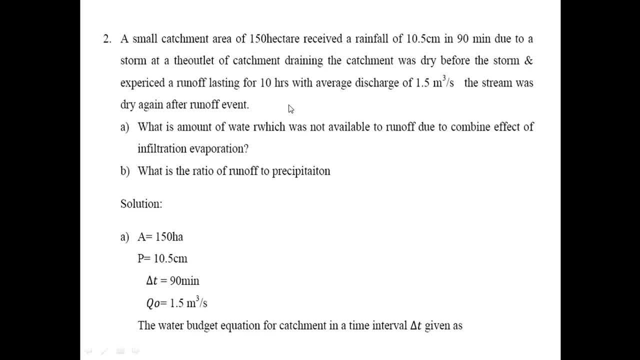 And the average discharge during the runoff is also given, which is 1.5 cubic meter per second, And the stream was dry again after the runoff event. First the stream was dry, After that there is a runoff in it. After the runoff is over, the stream is dry after the event of runoff. 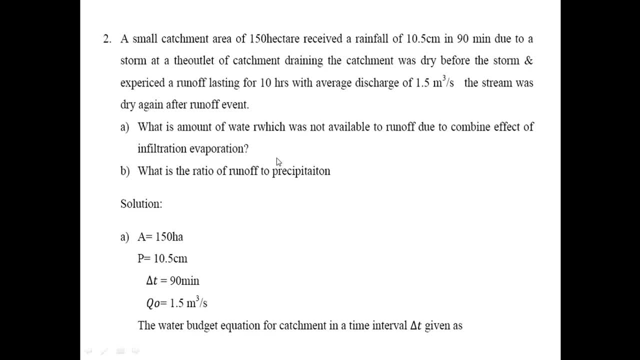 So, solution and solution, We will write the given data in given data. We have area given, which is 150 hectares. Precipitation is given 10.5 centimeters. Delta T, that is. time is given 90 minutes. Outflow is given, that is 1.5 cubic meter per second. 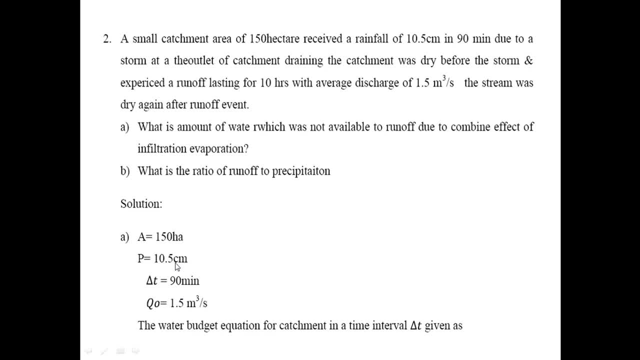 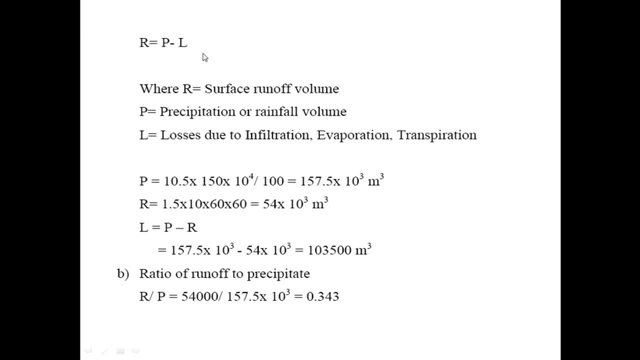 The water budget equation for a catchment area in a time interval, Delta T is given. as R is equal to P minus L. Here R is surface runoff volume, P is the precipitation rainfall volume And L is the losses due to infiltration, evaporation and transpiration. 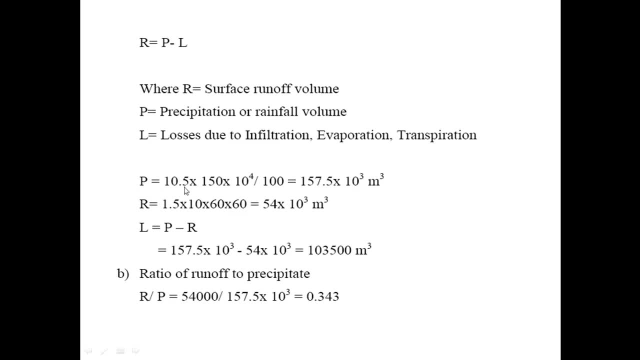 Here P is the total precipitation. that is 10.5 into 150, into 10, to the power 4 divided by 100. The total precipitation that we have is 10.5 centimeters. We have to convert it into meters. So 10.5 divided by 100 is the value of this. 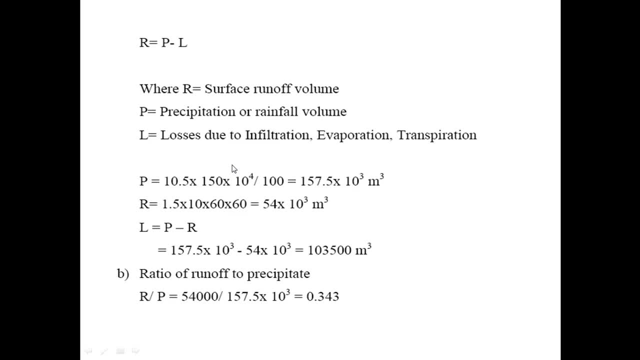 You have to multiply it from the total area, Because there is precipitation on the total area, So you will get the total at net precipitation or rainfall volume, That is, 157.5 into 10 to the power 3 cubic meter. This much amount of rainfall is the occur. 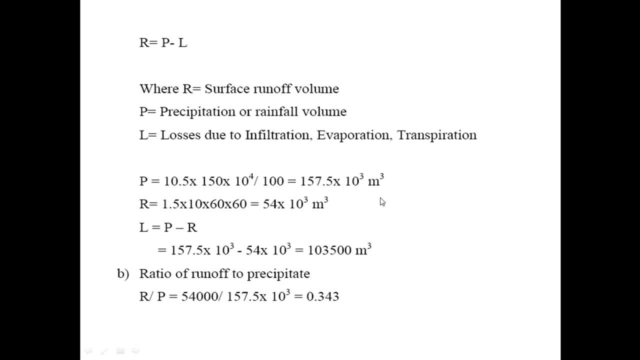 And this is the total volume of the precipitation or rainfall water. The losses are is sorry. The surface runoff R is equal to 1.5 into 10, into 60, into 60. Here the total runoff is 1.5 cubic meter per second. 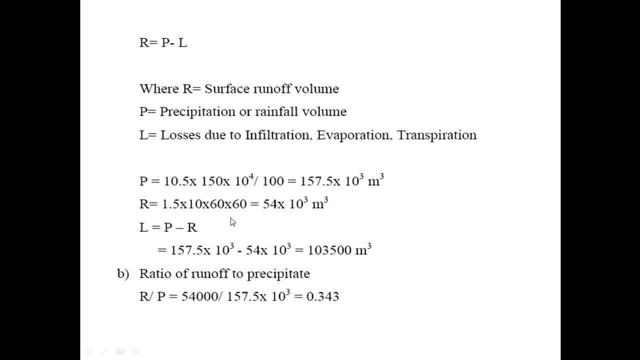 So the time here. multiply this value with the time, that is, 10 hours. Multiply this with 60 minutes. One hour have 60 minutes And also one minute has 60 seconds, So you will get the total surface runoff in cubic meters.